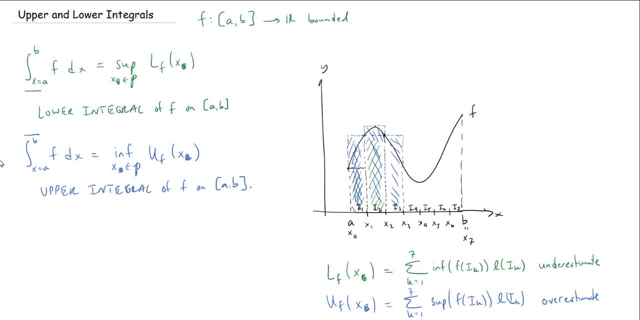 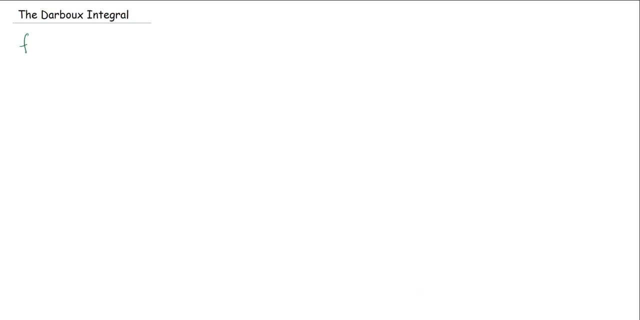 Let's say, if you like, the area under the curve, although that's not totally working, if f is negative or something, Okay, so let's set it up as before. We have our function f from a to b, and it's going to be a bounded function. 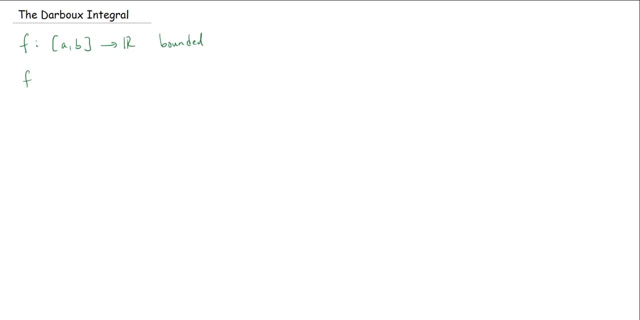 And so we're going to say, We're going to say that f is Darbeau, although we won't usually write Darbeau integrable. So integrable If well, we have this lower integral right. 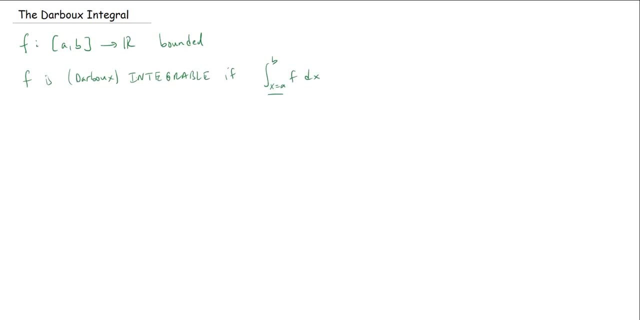 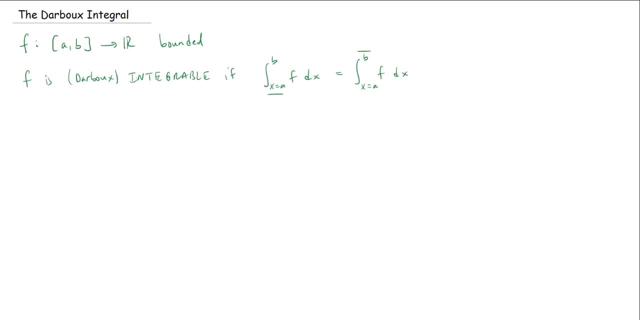 Okay, Okay, Are equal, then we say that the function is integrable, And in this case we denote the common value By the more traditional integral that doesn't have a bar on the top or the bottom. Okay, And so this is what we'd call the integral of f over the interval a- b. 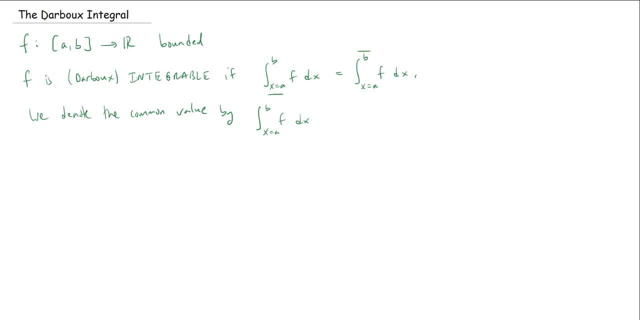 So there you go. so let's do an example now. we could do, you know, very straightforward examples with continuous functions. we're actually going to have a theorem that we'll do in a subsequent video, where we prove that any continuous function on an interval like a, b, is going to be integrable. but let's take a. 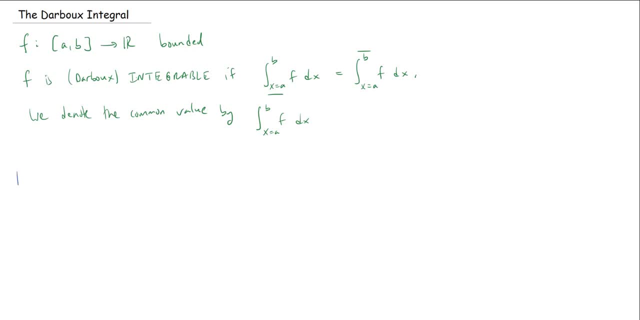 function that's not necessarily continuous, at least not everywhere. so i will go back to one of my favorite functions. it's a piecewise function. it is three or one, depending on if x has gotten to seven yet or if it's past seven. okay, so if we draw a picture, 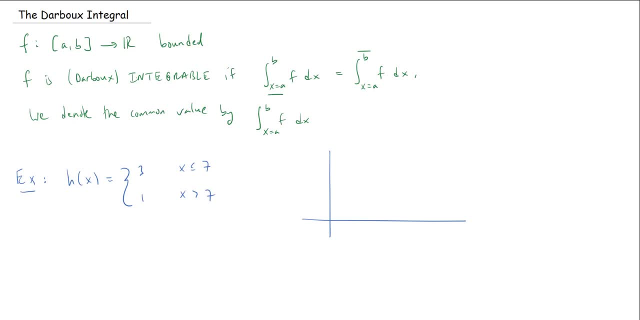 so let's see, we'll put seven about right there. so the graph: before you get to seven, you're up here at three and then once you get down to seven, or once you get seven, it goes down to one, like: so okay, so there could be our x and 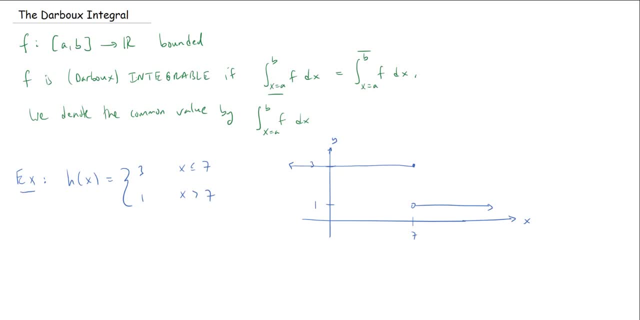 our y and let's say that i'm going to restrict the domain to the interval five to ten. all right, so i can jump in here and is all right, five, maybe it's going to be about right there. ten is going to be over here and i would like to know. 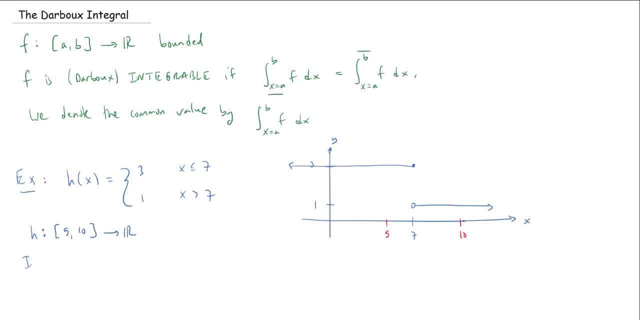 if H is integrable, all right, so is H integrable, okay. and the problem from the point of view of the function right is that there's this big discontinuity right in the middle. but from sort of an intuitive point of view, we shouldn't really be too surprised that this was integral, because look, if I want to. 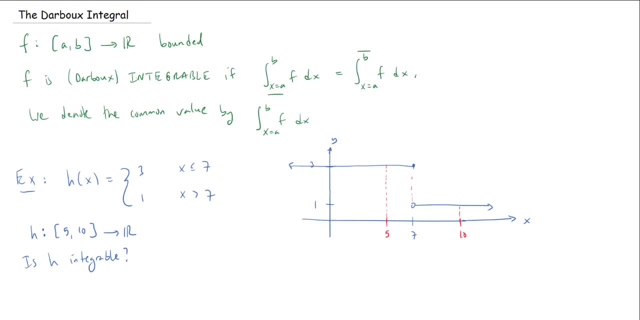 integrate from 5 to 10. what I should be asking for is: can I compute the area under the line and? and: yeah, right, like yeah, even though there's this little discontinuity, it's still pretty easy just to build these two, two rectangles up, alright. so this first one has height 3 and base 2, so this should be 6. this. 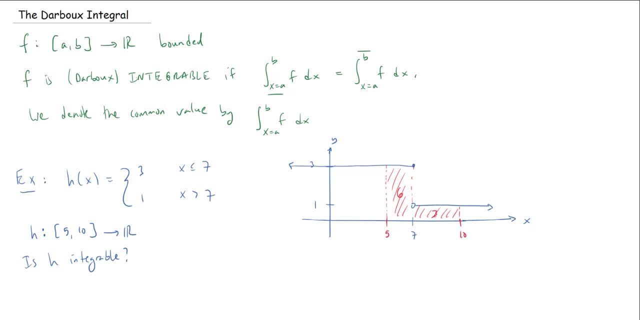 has height 1 and base 3, so this should be a 3. so what should be the case, so we expect, is that if we integrate from 5 to 10 this function H, that we should get 9 right, 6 plus 3, all right. all right, but let's go through the actual definition. 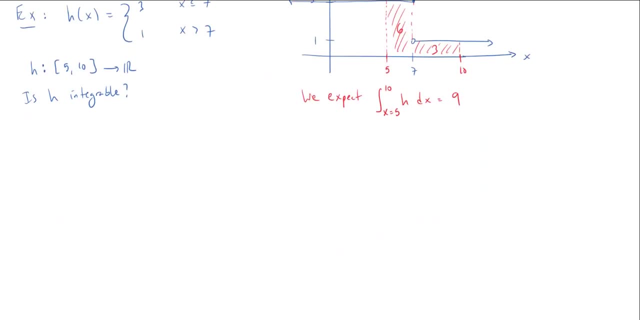 all right, let's see if this, this really works. so first thing we're going to do is we're going to define for any positive integer, say little n. I'm going to define a partition, so we're going to let x and I'll put the n up here. it's not an exponent, okay, I'm not raising. 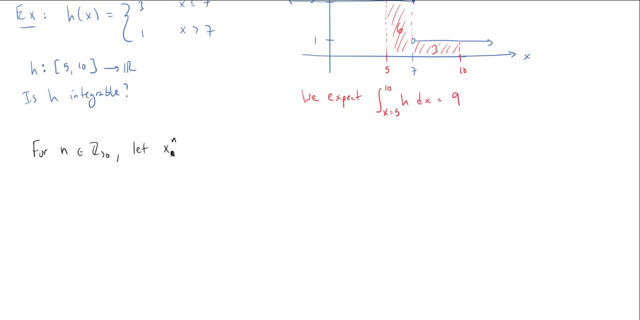 this to the nth power. I'm just, it's just a place to put an index, okay, and so this is going to be the partition that starts at 5, and then it's going to go to 7 y 7. well, that's where this little discontinuity occurs. then I just do a 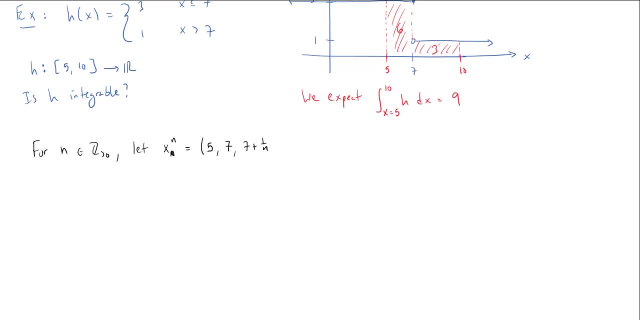 teeny little jump to the right: 7 plus 1 over n. when n is very large, then of course 7 plus 1 over n will be very, very close to 7. okay, and then I'll go to the end of the interval: 10, okay, and so this should be. this was a partition, in fact we could. 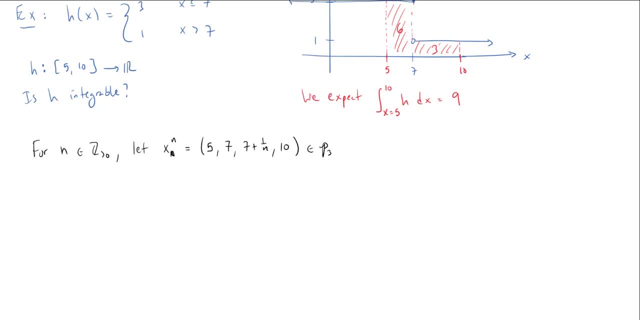 see right. there's three commas: 1, 2, 3. so this is a 3 partition of the interval 5 to 10. all right, now, since I'm trying to show that H is integrable, I need to show that the lower and the upper integrals. 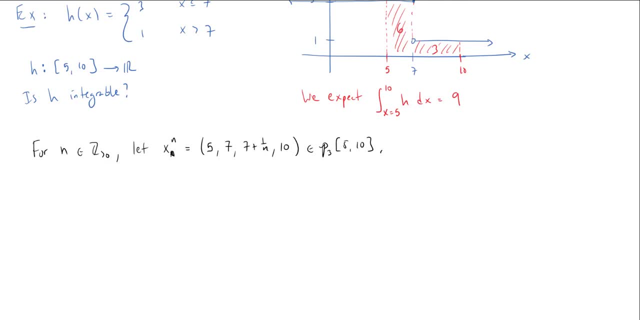 are equal, but each of those is defined in terms of lower sums and upper sums. so let me compute the upper sum for H here, so the upper sum for H on, say, this particular partition X, n. so what I need to do is for each of these intervals. 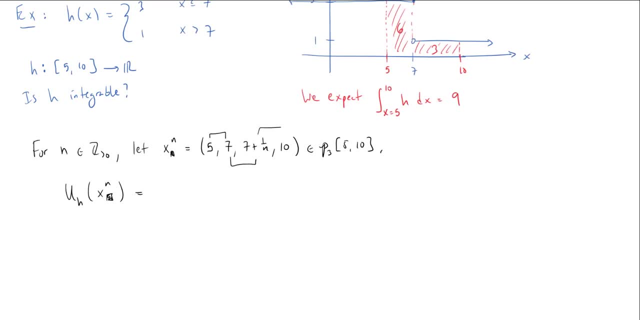 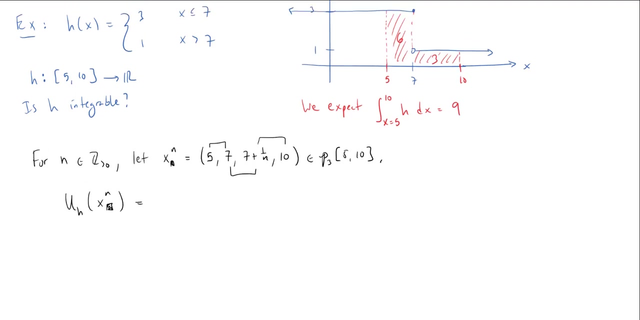 okay. so there's one interval, there's a second interval, there's a second interval, there's a third interval. I need to compute the supremum of the function H on that interval times the base size, right. so between 5 and 7, the supremum of. 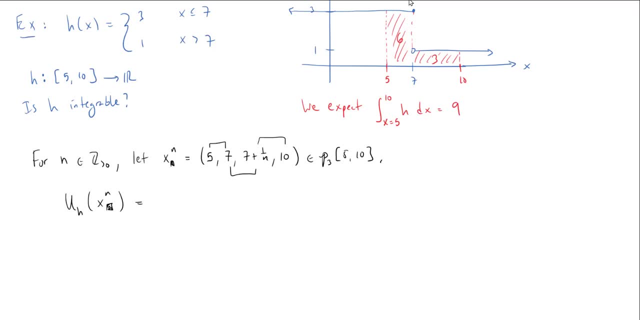 H. well, actually H is constant from 5 to 7, right, just as height 3, so this will be 3 times the width. okay, well, the width from 5 to 7 is 2, all right, plus now we go to the next bit. all right, so here I'm going to have some 7 plus 1. 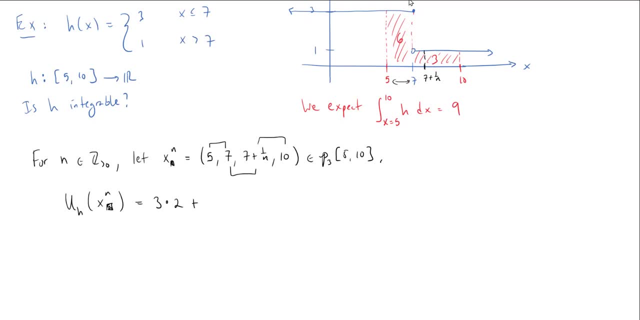 over n. and on this interval, where is the the supremum? well, at first glance you might say, well, it's 1, right, that's everything on this interval is 1, but actually, remember, we get to include 7, and that 7, the height is still 3, so I 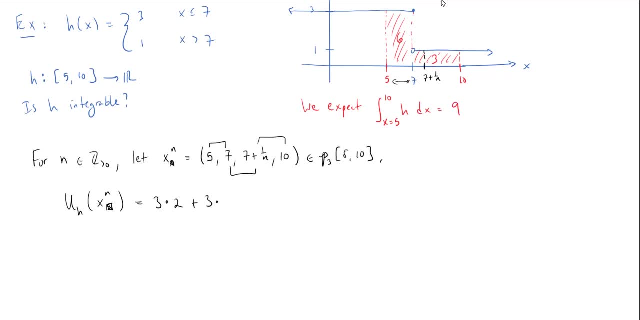 still get a 3 as my supremum times. the width, well, from 7 to 7 plus 1 over n, the width is just 1 over n. okay, now we go to the last piece, that's from 7 plus 1 over n to 10, and again, it's not hard to. 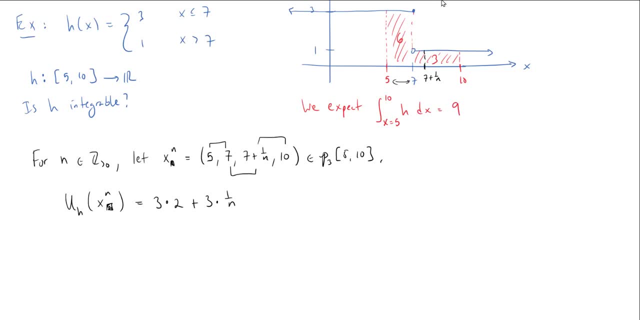 see what the supremum is right, because it's just constant everywhere on here. the supremum is just going to be 1, so plus 1 times all. right. now, how far is it from 7 plus 1 over n to 10? well, from 7 to 7 plus 1 over n to 10 is just 1 over n to 10, and again, it's not. 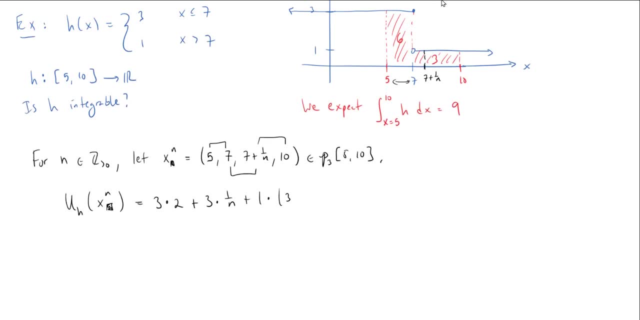 that fast recorded here. so somewhere here in your mind it's still 1. and then here's the first step: only when you error. alright, let's continue. so 7 to 10 would be 3, but you're not starting at 7, you're. 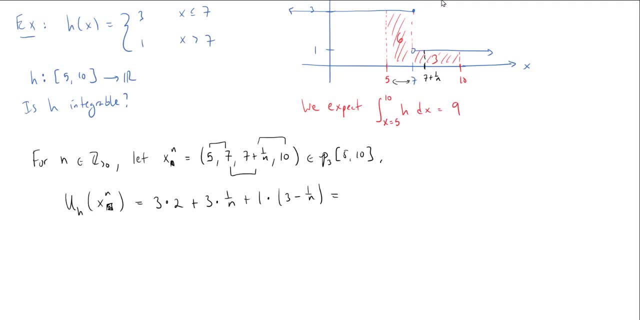 starting 1 over and over, so we have to subtract 1 over n. okay, let's see we can put this all together and all right. I have: 3 times 2 is 6 and 1 times three is three. so six plus three is nine. then I have three times one over n and one rate. 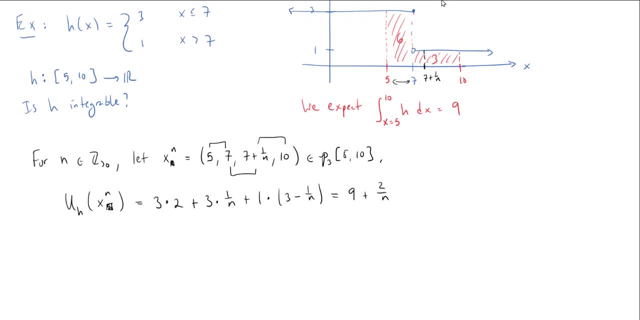 over n. Ah, so the upper sum for this particular partition is given by 9 plus 2 over n, and we see pretty easily, right as n gets large, this is going to converge to 9.. Okay, so this. we'll just keep that in the back of our minds. Now let's try to compute lower sums only this time, instead of using 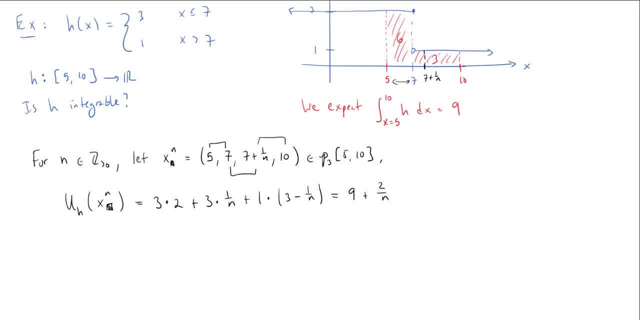 this xn. I'm just going to actually pick a very specific partition. that's even easier. So let's let w. this is just going to be the partition that doesn't even have this extra 7 plus 1 over n, but I'll just go 5, 7, 10.. All right, so this is now just a 2 partition of 5- 10.. 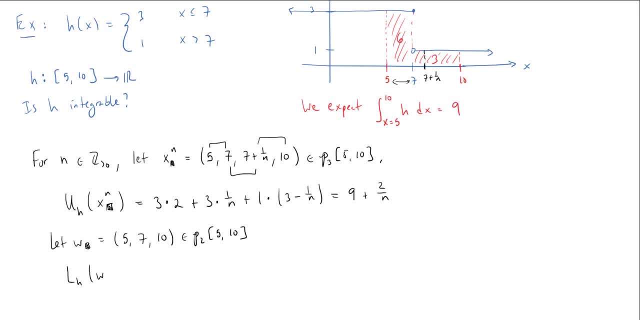 And let me compute the lower sum for w. Okay, well, let's see. so, between 5 and 7, the infimum, well is, it's just a constant function, right? so the infimum is the supremum is just equal to the value of h. so this is still 3, and the width: 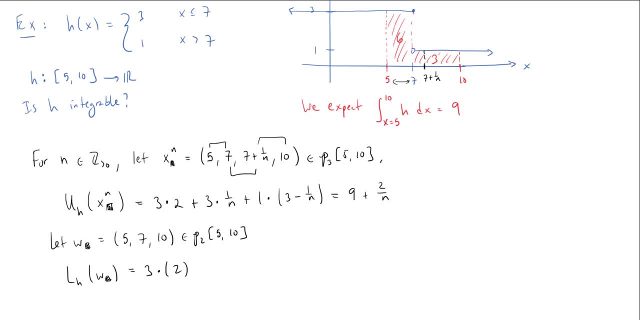 is still 7 minus 5, which is 2.. Okay, then we go to 7 to 10. right, there's just two of these now, and from here we're going to get the lower sum. So we're going to get the lower sum. So we're going to get the lower sum. So we conclude that the lower sum is equal to 9.. 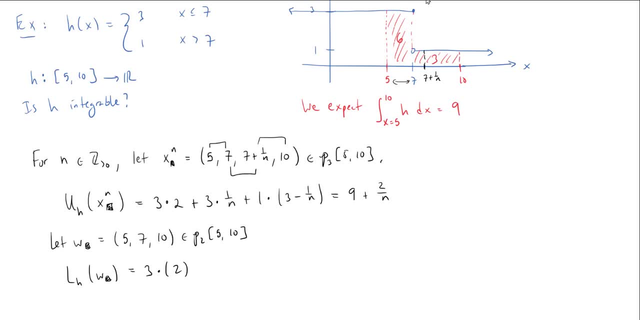 Well, the supremum was 3, because you had this one point at 3, but if I'm doing the infimum, I don't worry about this 3 up here I get all these 1's. that's the infimum, So it'll be plus 1 times. now, from 7 to 10, that has a distance of 3.. 3 times 2 is 6 plus 1 times 3 is 3.. Okay, 6 plus 3 is 9.. Ah, so we conclude that the lower sum is equal to 9.. 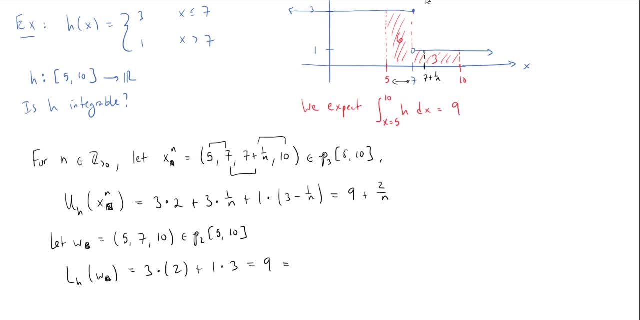 But this lower sum that's actually equal to the infimum of all of these upper sums. All right, so if I let n range from 1 to infinity and I look at all of these upper sums, then of course I'm getting all of these expressions of the form 9 plus 2 over n. 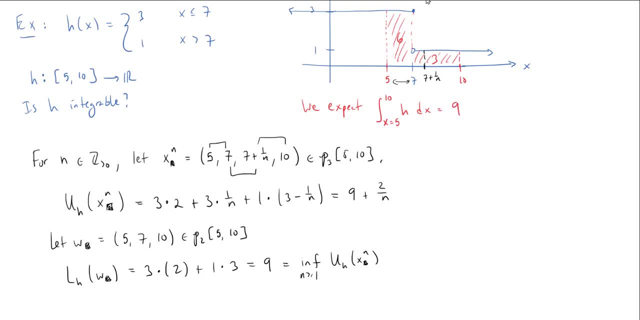 and the infimum of this expression is 9. itself Okay, but the infimum of all the upper sums is equal to the upper integral. So this is the upper integral of h, dx, Ah, so this particular lower sum is already equal to the upper integral. 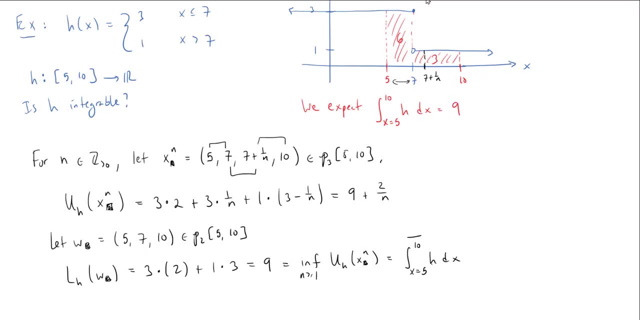 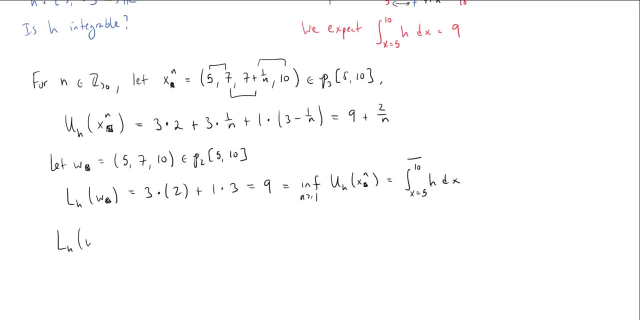 And I know that the lower integral is the supremum of all of the lower sums. All right, remember this. So l h is certainly, or at least of w is going to be well here. let's write this first with. we'll write the upper integral first now. 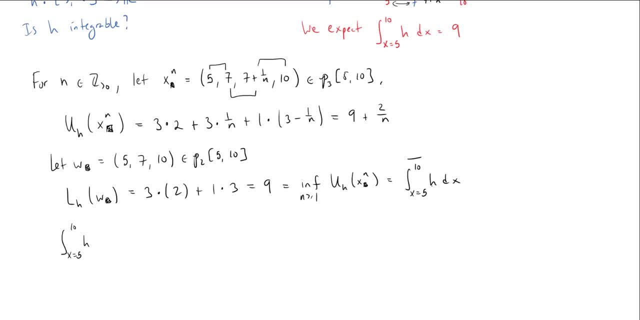 So the upper integral is equal to this lower sum of w, But the lower sum is certainly equal to the supremum of all lower sums. So if I say, take an x here and let x range over all possible partitions, well, maybe I won't use x. 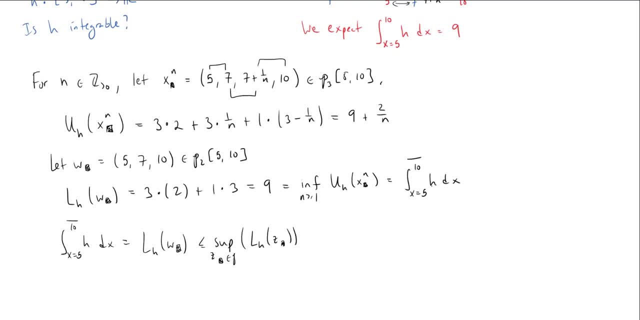 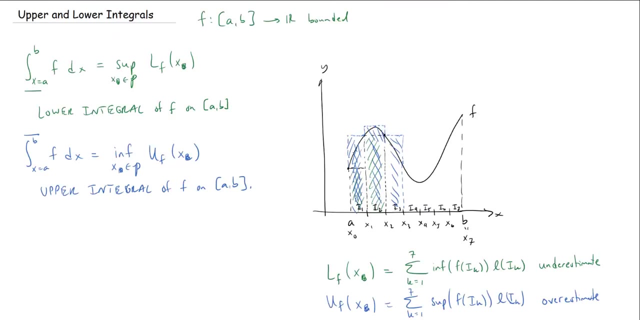 I'll use z, because we's x up above, so I'll use z. So, if I look at all of these things, but this supremum is equal to the lower integral. Okay, but in the last video we showed that lower integrals are always less than or equal to the corresponding upper sum.